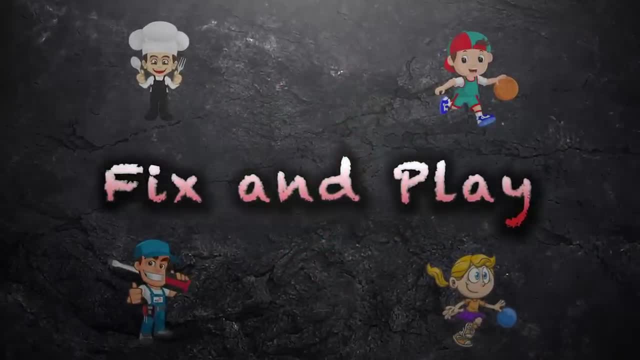 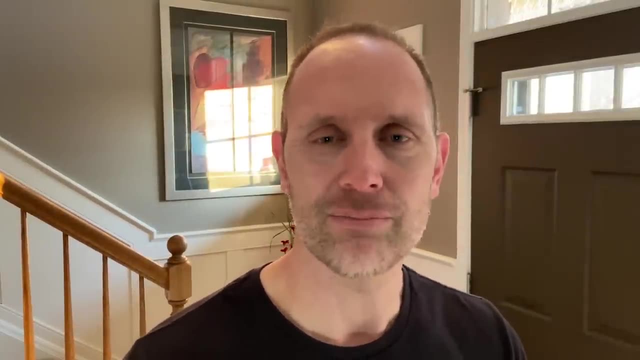 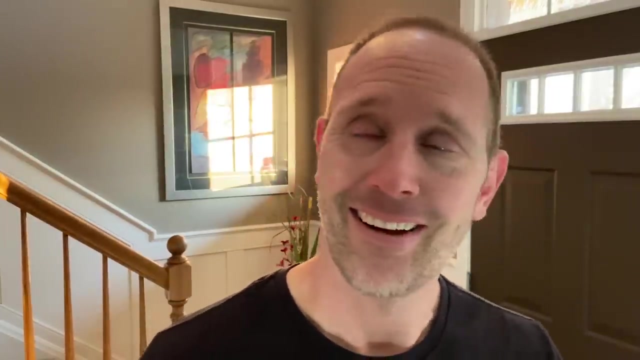 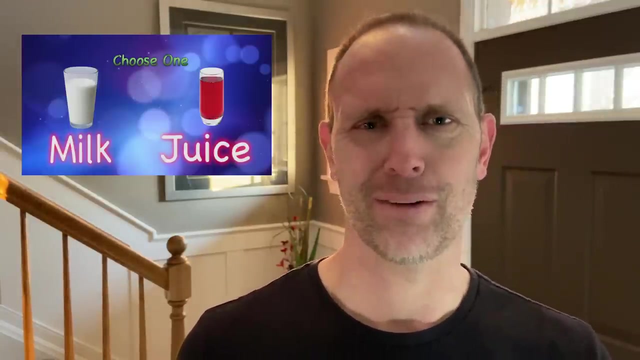 Hey everybody, You want an activity to get your kids moving and put some variety in exercising. Well, I got it. It's called: Would You Rather Workout? Here's how you play. All right, Would I rather have milk or juice? For sure it'd be juice, Not even close. Okay, so now I do the 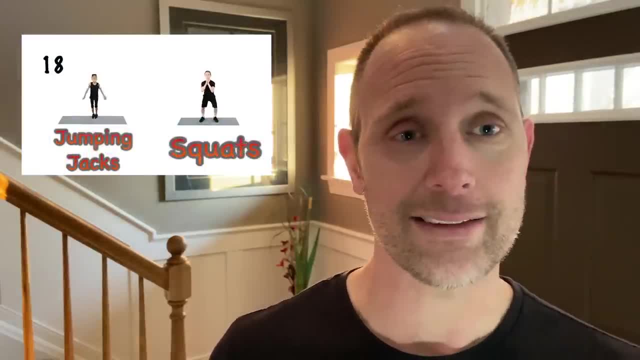 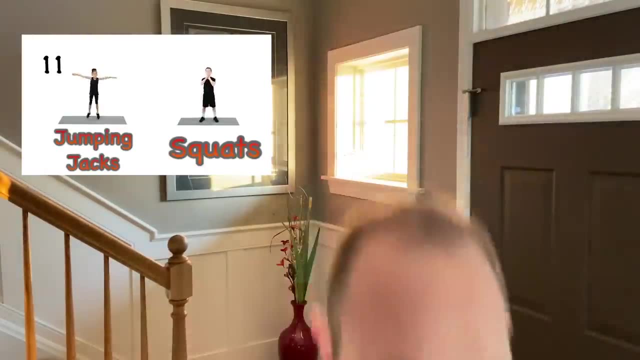 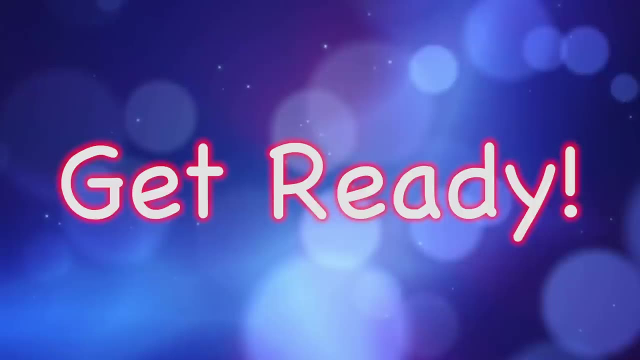 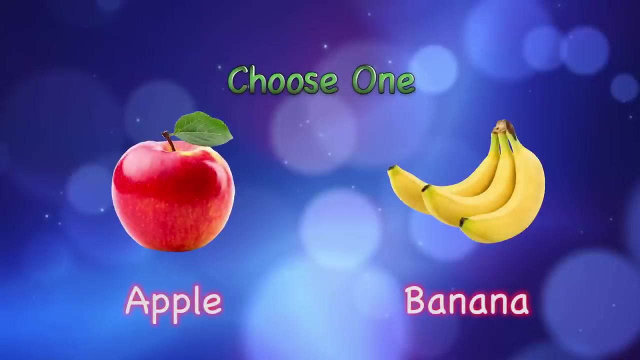 exercise that goes with juice. Looks like it's squats. All right, I think you get the idea. See how easy that is. Okay, great, No problem, All right, Hello, we're not ready to start working. Oh, she's not ready. 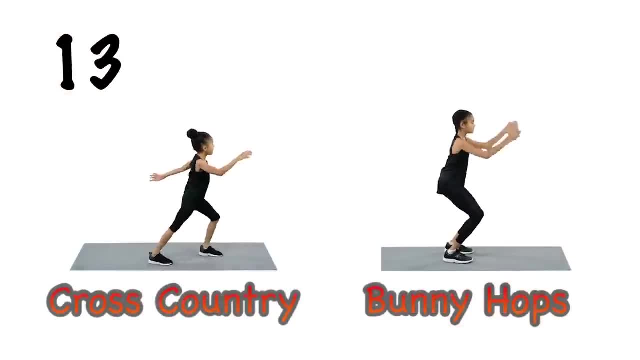 Just drill down a bit. Okay, It's gonna be a hard one. Okay, One more time. one more time, One more round. Okay, I'm gonna do the same thing. It's gonna be an exercise that I would do. 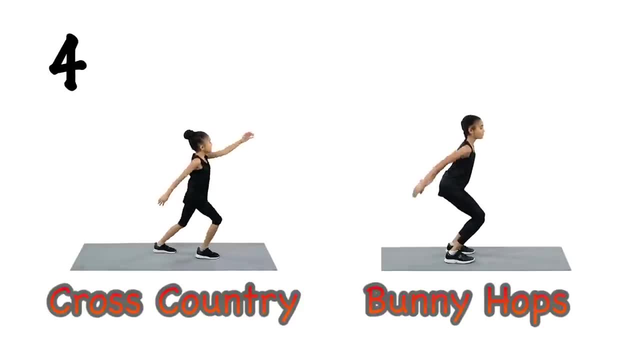 Please don't believe you're learning. I'm not even gonna do it. Yeah, it's okay. I'm not even gonna believe you're doing it. It's okay, I'm not even gonna do it. Okay, You know what I'm saying? 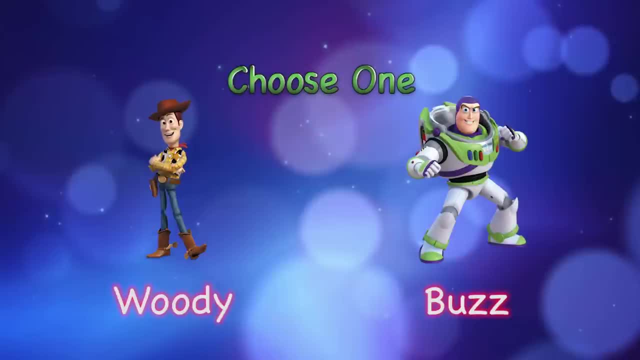 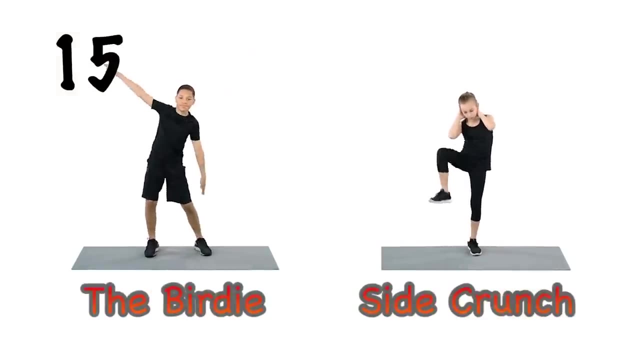 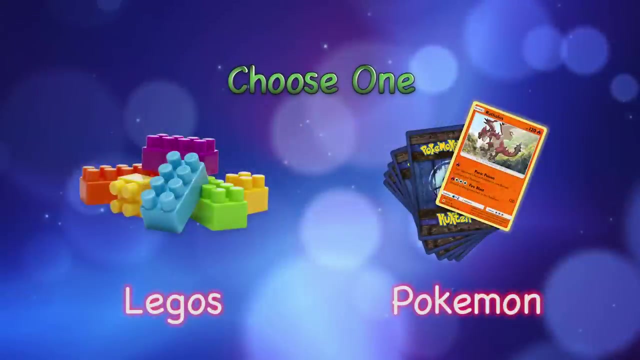 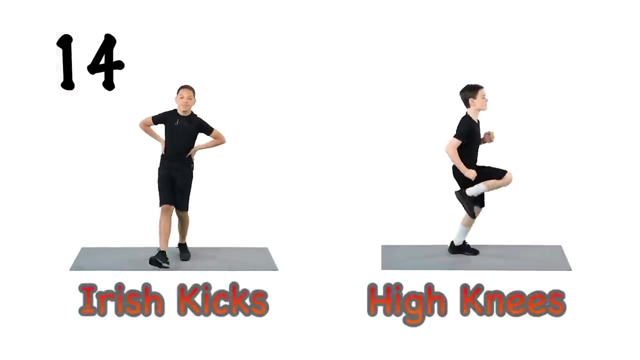 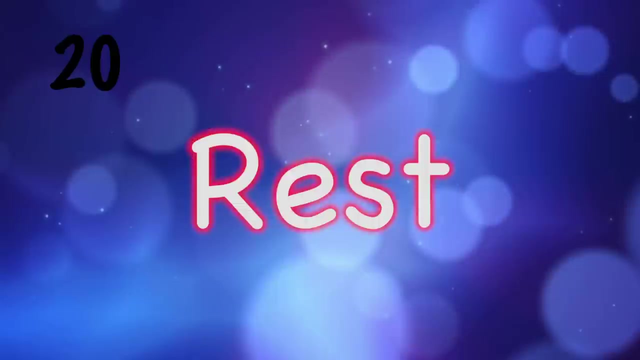 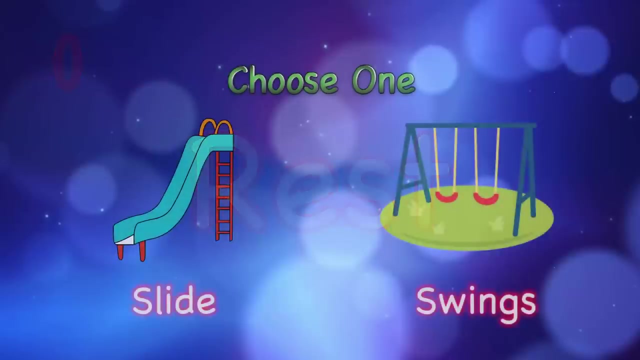 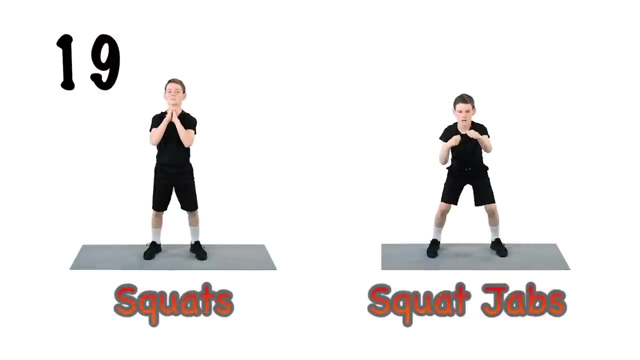 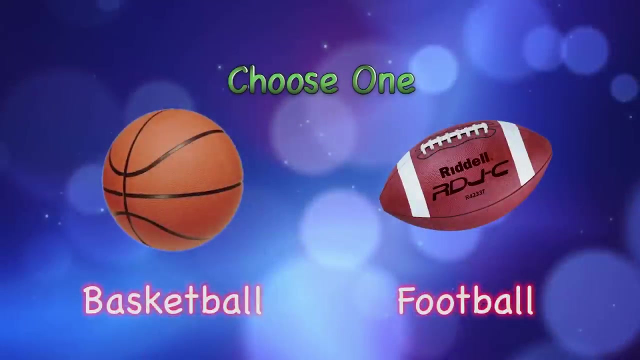 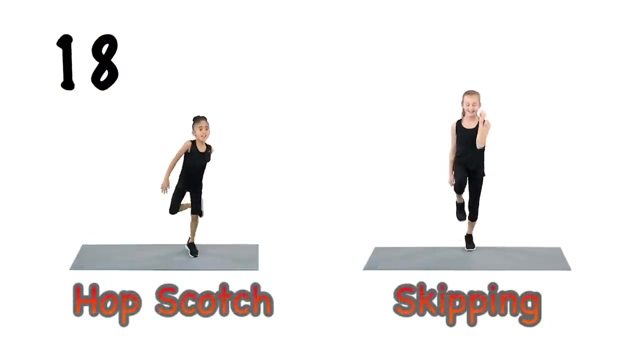 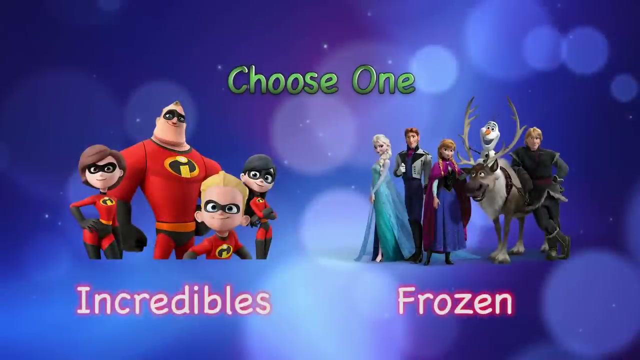 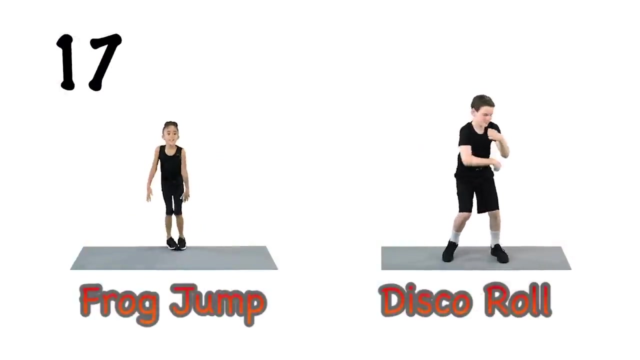 I have something I haven't done in a while. I'm just gonna do it. I just wanna do it. You know what I'm saying. We'll see you next time. Bye-bye, Bye-bye, Bye-bye, Bye-bye. 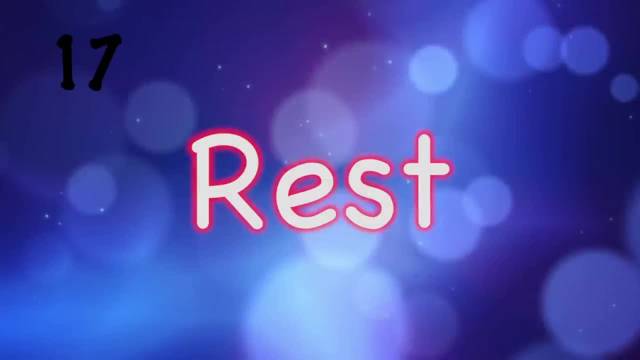 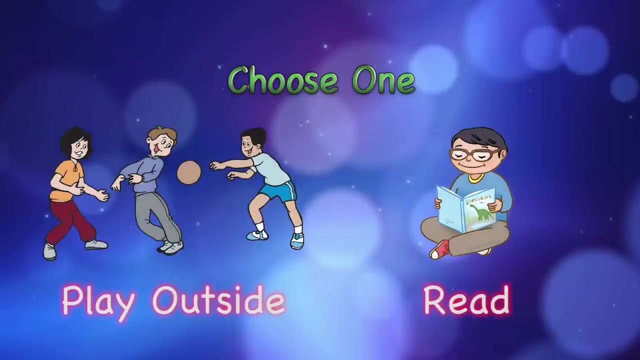 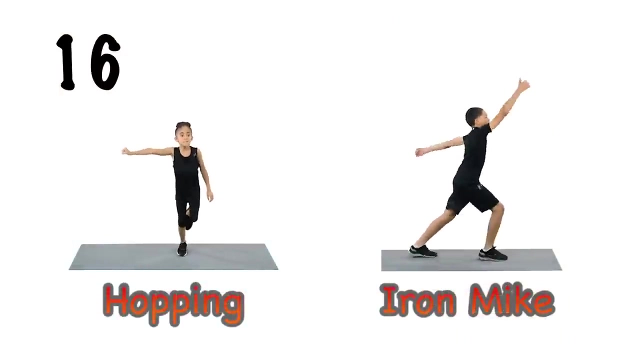 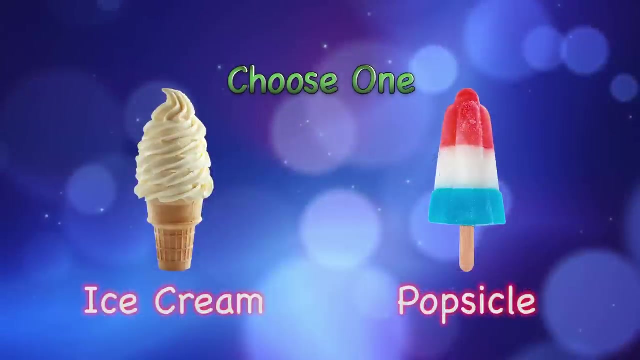 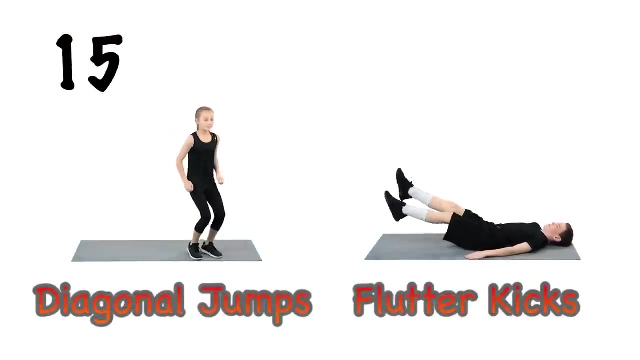 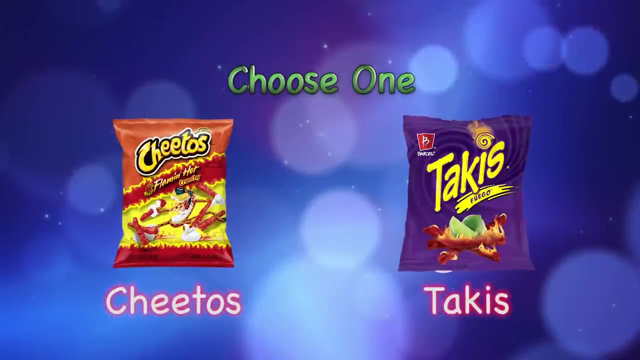 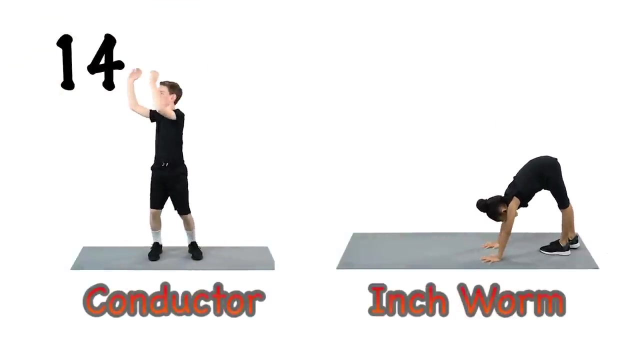 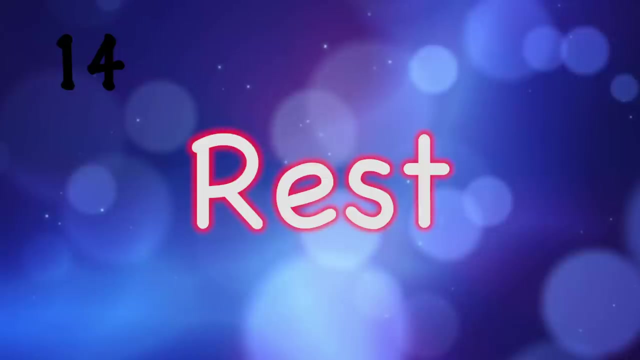 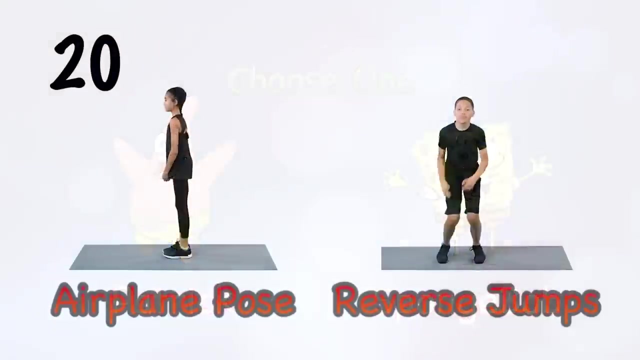 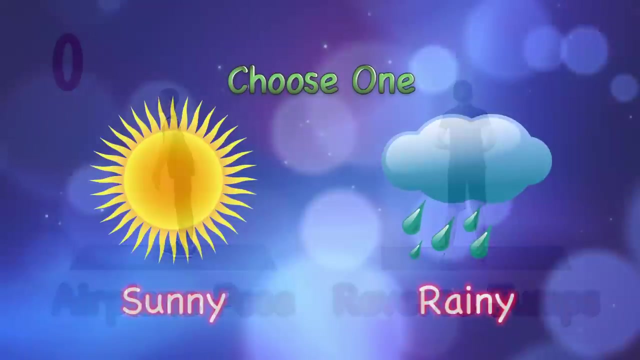 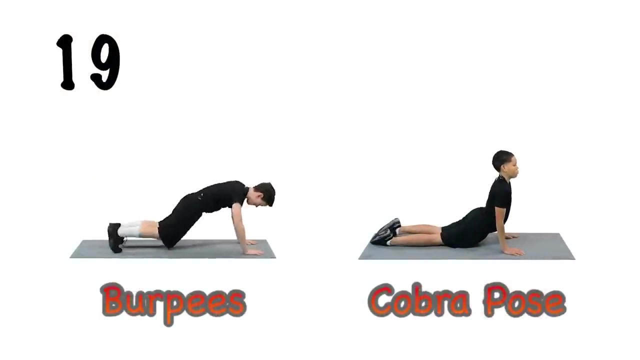 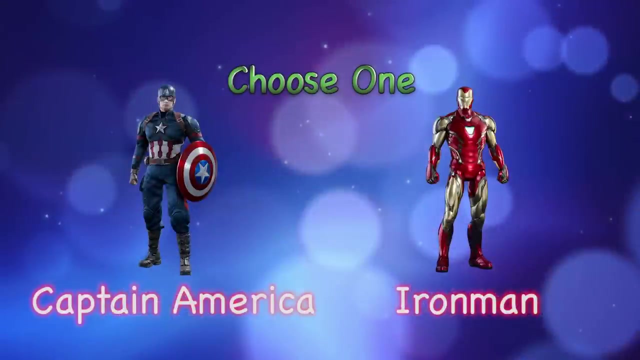 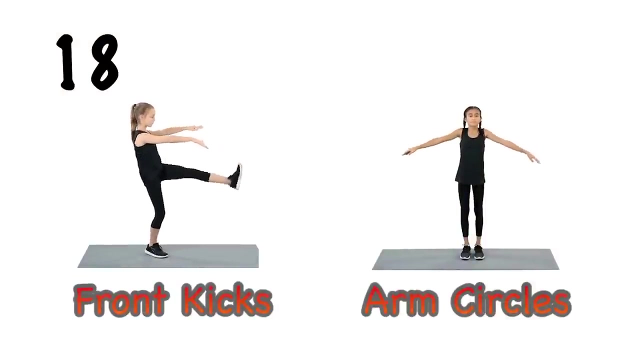 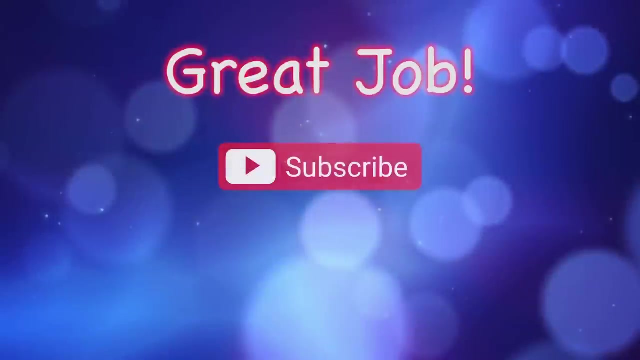